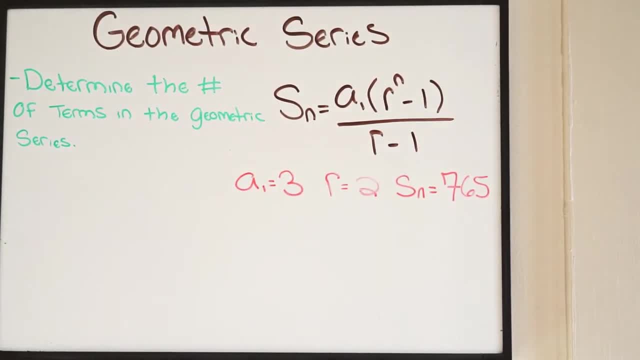 Okay, so, moving on with geometric series, we're being asked the following question: They want to know determine the number of terms in the geometric series. So, again to the right, here we have the equation we use to calculate the sum of a geometric series, And we're actually 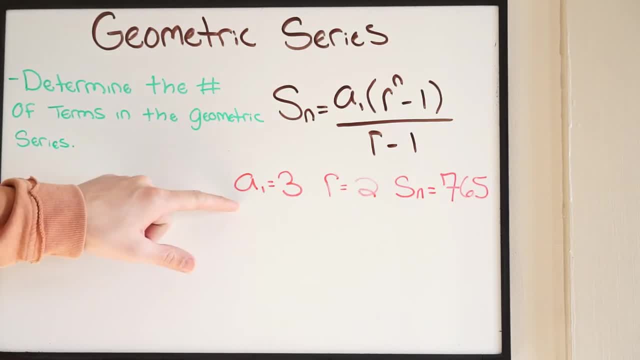 provided the values here. So again, a of one that's going to be the first term in our geometric sequence, R is going to be our common ratio in our geometric sequence, Okay, and s of n. this is going to be the sum of the geometric series, Okay. so what they want us to do here? 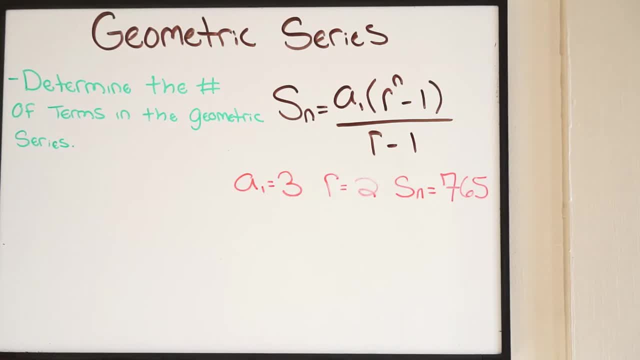 is, they want us to find the number of terms in this geometric series. Okay, so let's talk about how we're going to determine this. Our first step is: we need to use our equation here for geometric series And we're simply just going to plug in our known values here. Okay, so we know. 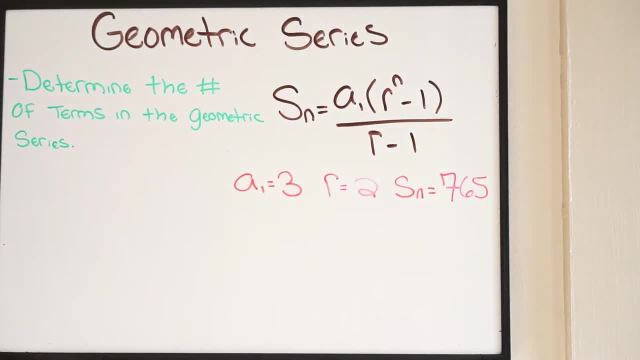 that the sum of the geometric series is going to be 765.. So let's fill that in So we have 765, equal to now. our first term is going to be three, so a of one is three. Okay, our common ratio is going to be two, And then we just have n here. that's what we're solving for, right This. 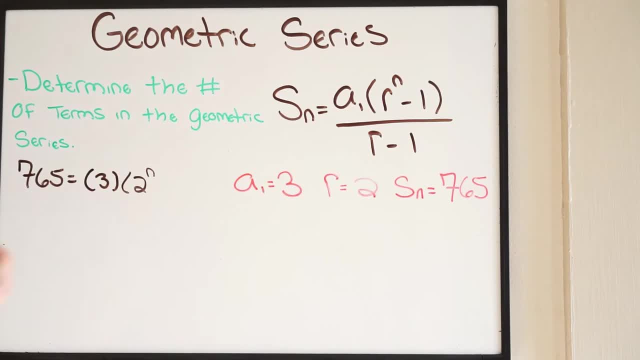 is going to be the number of terms, Okay, and then we're going to have minus one, Okay, and then we're going to have two minus one, Okay. So let's go ahead and clean this up. Well, we know that two minus one is simply going to be one. 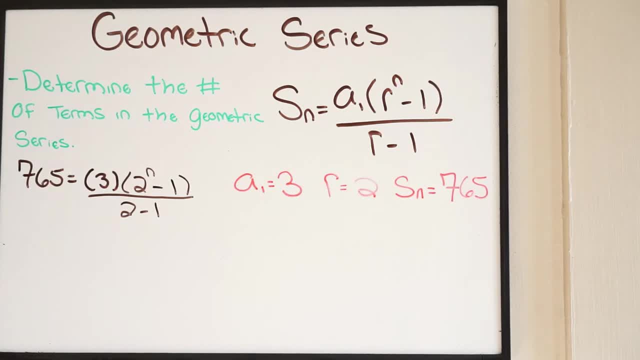 And anything divided by one is just going to be itself, right, So we can just go ahead and rewrite this as 765 equal to three, And we have two to the n minus one. Okay, at this point we want to go ahead and divide both sides by three. Okay, so that will cancel. Let's go ahead and plug this. 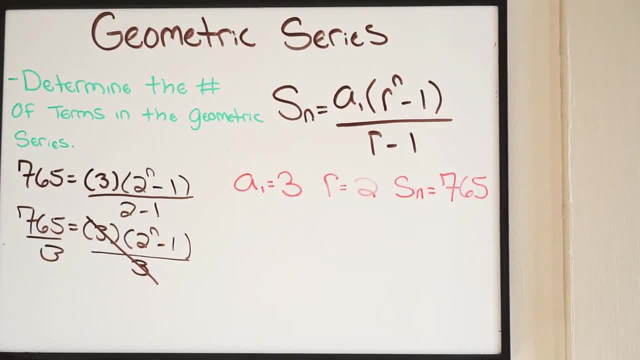 into our calculator. So we get 765 divided by three and we get 255.. So we get 255 equal to two to the n minus one. So let's go ahead and get rid of this negative one. we're going to add one on both sides. So now we